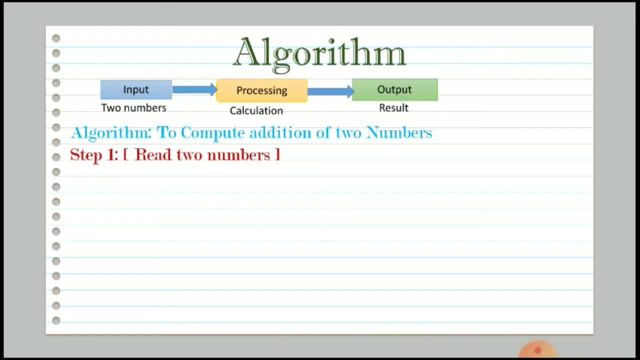 is the second number, then the statement to read these two numbers will be read: n1 comma n2.. Now in second step we already know what the input is, that is n1 and n2 is our input. So now we have to perform addition of these two numbers and that result will have to store. 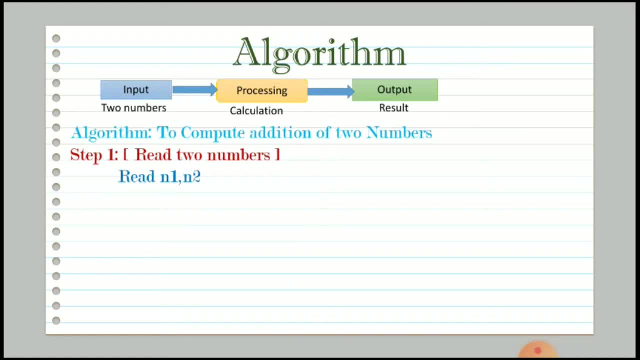 somewhere, Suppose we will store that result in sum. So in step two we will write this statement: add the numbers to compute sum. So again this statement, that is, add the numbers to compute sum, is optional. Then the next statement to make addition will be: 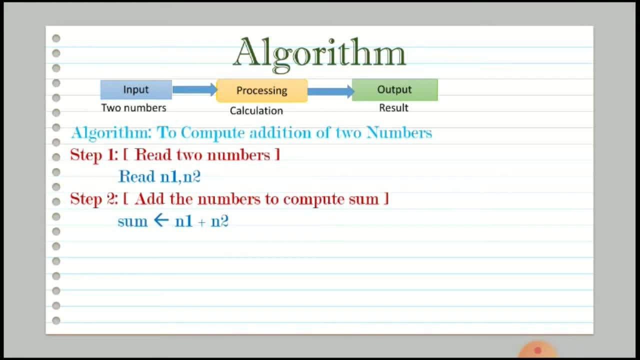 sum. So this statement indicates that n1 and n2 will be added and the result will be stored in sum. So till now we have taken two numbers as input in first step. In second step we have processed these numbers. that is, we added these two numbers and the result we have stored in sum. 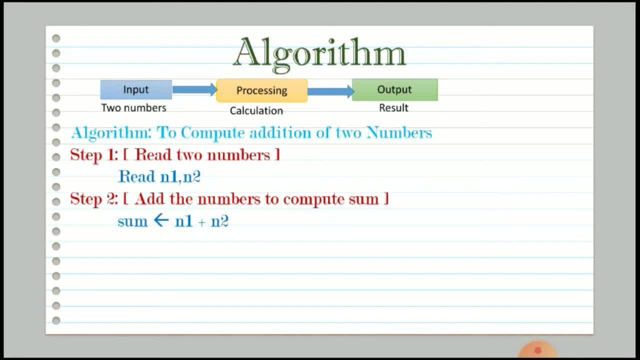 Now, in step three, we have to display the output. So in third step, we will write the statement, print the sum. And even this statement is optional. You can write this statement or you can skip. Then to print the output, we will write the statement, add the numbers to multiply into sum. So we have to print the output and print the sum. 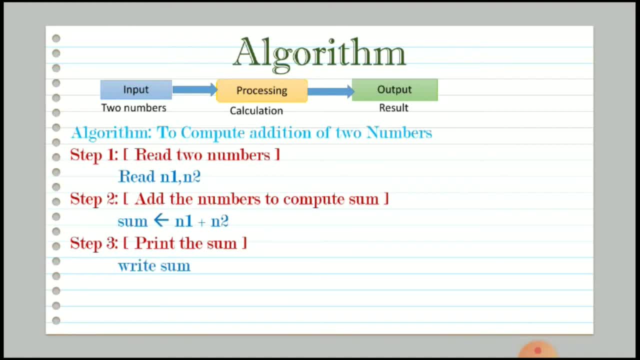 write sum. so after getting the output, our algorithm should be stopped. so the fourth and final step: we will write to stop the algorithm so we can write this statement: end of algorithm. again, this statement is optional. we can write or we can skip this statement. then the next statement we have to write: either stop. 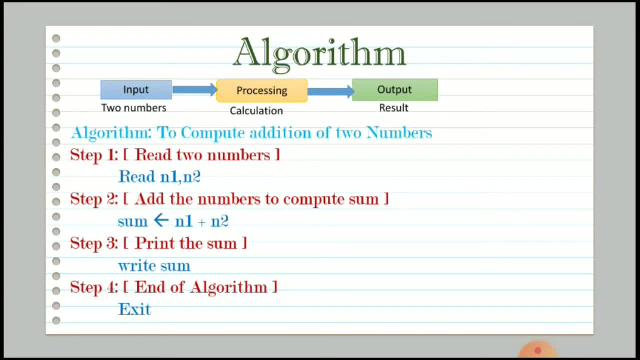 or exit. so whatever we wrote in square bracket is optional in algorithm. you can write that statement or you can skip that statement. this statement written in square bracket is jut to understand what is divisible by a variable and say: whatever got written in square bracket is just to understand what is. 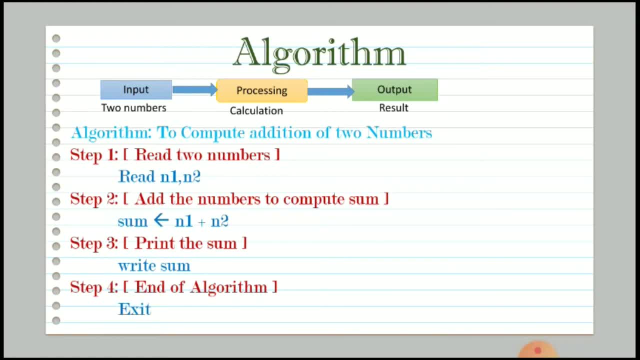 happening in that particular step. so the same algorithm. you can write it as: in first step we are taking input, that is, we are reading two numbers, n1 and n2. then in second step we are adding n1 and n2 and then that result is stored in. 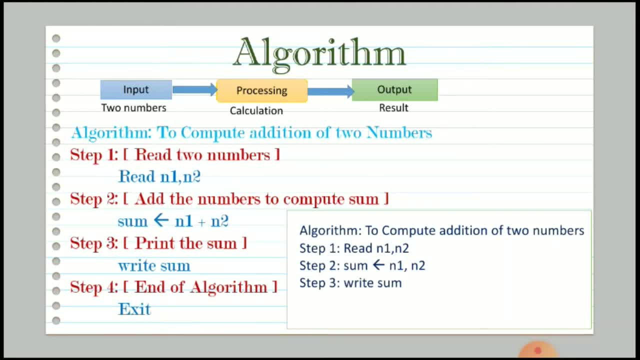 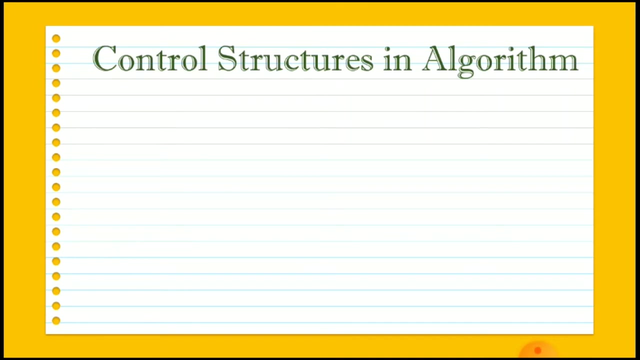 sum. in third step we are printing the output, that is, write some or you can write print sum. and last step: we have to stop the algorithm. so you can write either stop, oh or exit, so you can choose either the first format or second format. so now we 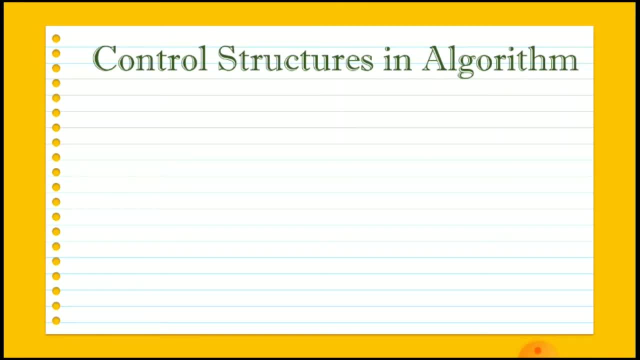 will see control structures in algorithm. so there are three types. first one is sequencing, second selection and third repetition. so in sequencing all the steps which we write will be executed one after another. that means if there are five steps, then here first step will execute first, then after executing step. 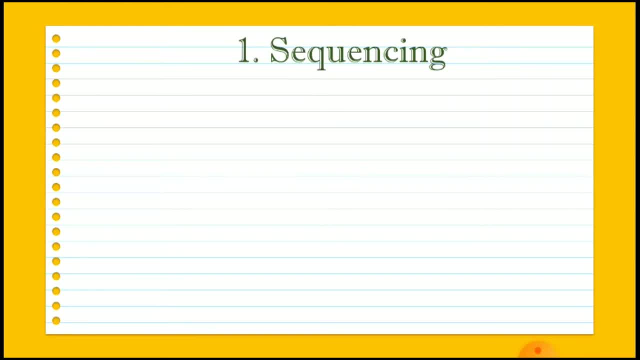 first. second step will be executed, second step will be executed, third repeat: executed. and like that, each step will execute one after another till the last step. So basically, here control of algorithm will be in sequence. The second type is selection. In selection in a particular position depend on condition, one step will execute and another. 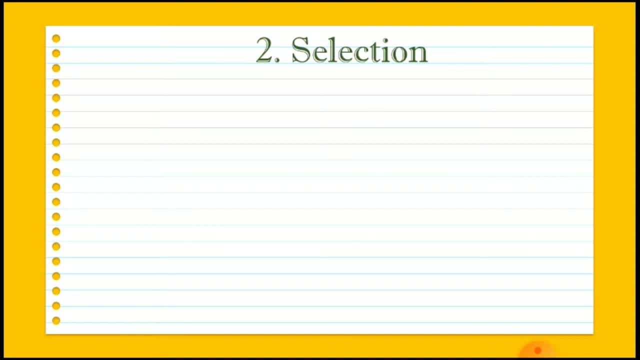 step will be skipped. That means, suppose, if there is condition and depend on condition whether it is true or false, one step will execute and other step will not execute. So suppose after executing first step There will be condition- depend on whether condition is true or false, step will execute. 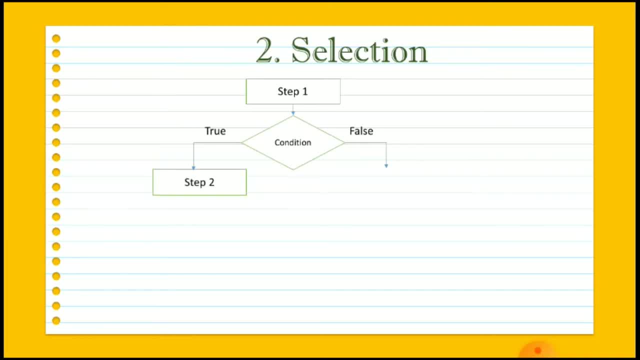 Suppose condition is true, Then step two will execute and step three will not be executed. and suppose condition is false, Then Step 3 will execute Right and step two will not be executed. after executing either second or third step, next fourth step will execute and then the remaining steps. 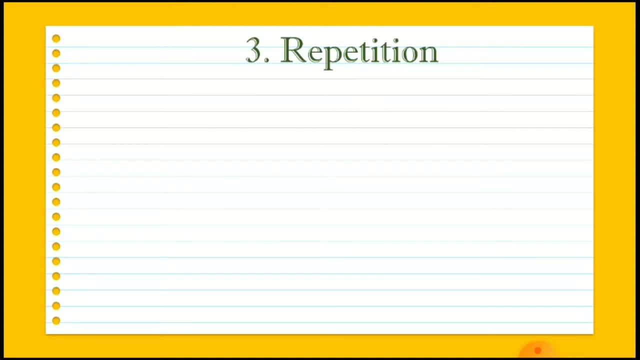 the third type is repetition. in repetition one particular step will execute continuously till the condition is true and once that condition becomes false, that particular step will stop executing and remaining steps will start executing. so suppose, after executing the first step there is condition. depend on whether condition is true or false. 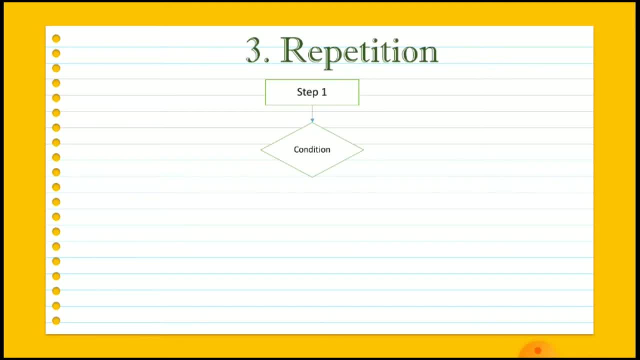 a particular step will execute this particular step. in this example, step number two will execute continuously till the condition is true. once the condition becomes false, it will stop. so the first step will start executing the second step and it will go to the step three and after executing third step, remaining step will be executed. the name given: repetition because 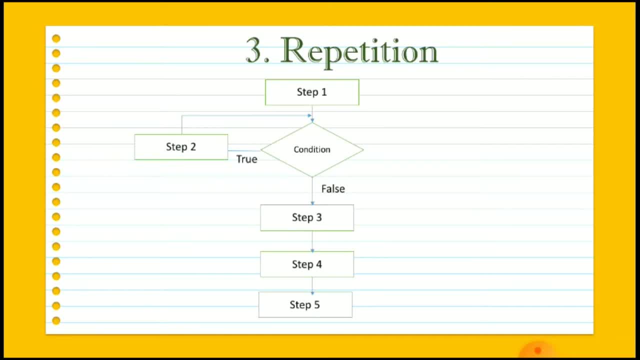 a particular step will execute repeatedly depend on condition. so the first form is sequencing algorithm. so in a sequence of steps, the- this appears next- we can consider as sequence of steps in which sequence method followed in the third steps. algum step will start executing the second step after another, then the second step, then 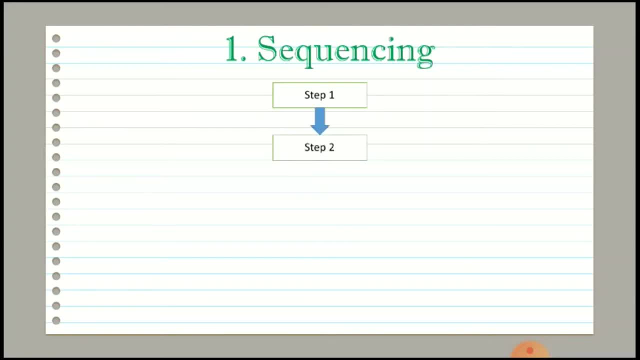 the third step after the third step will start executing the third step in order to see this pregnancy and in here, first step will execute first step after the second step and the fourth step will execute first step after the previous step will start executing the left step and then levanted blows will be executed in sequence. 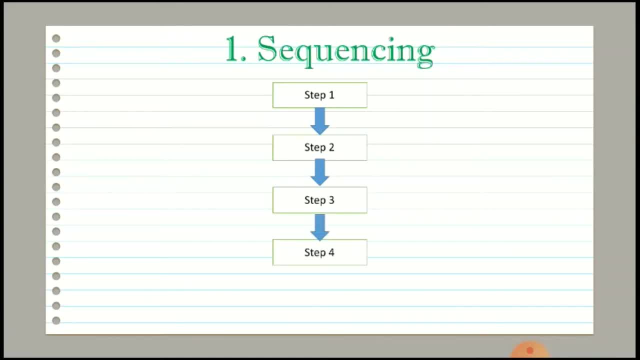 then the third step and so on till the last step. To understand sequencing algorithm easily, we will see one example Algorithm to find the total and average of three numbers. So, as you know, every algorithm is used to take some input and after taking input, we 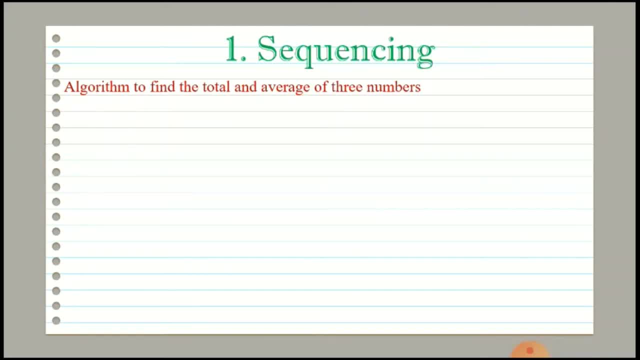 have to process that input and after processing input we will get the required output. So in this problem, three numbers will be our input, calculating total and average of three numbers. This is the processing part and the result that we will get will be the output. 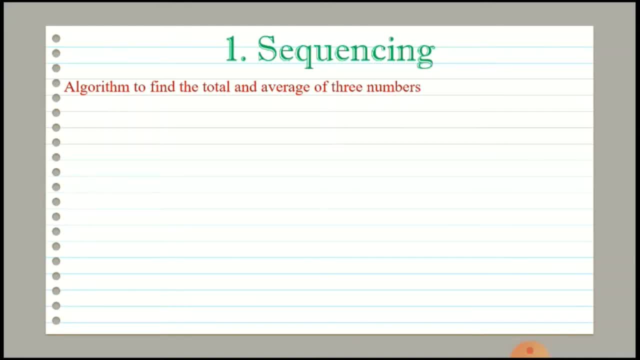 So in algorithm first we have to write the title of the problem, that is, to compute total and average of three numbers. Then in the first step we have to take three inputs. So suppose n1, n2 and n3 are the three inputs. 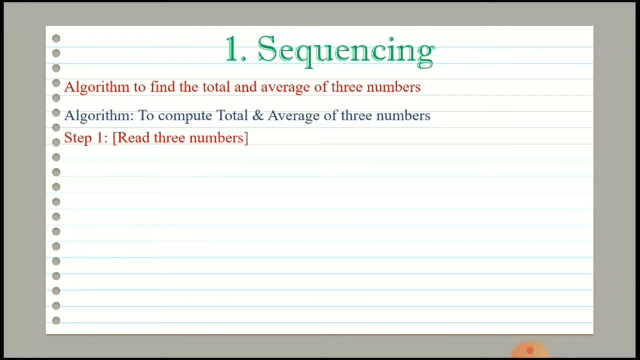 So in the first step the statement will be read: n1 comma, n2 comma, n3.. So instead of n1, n2 and n3 you can take anything like first number, second number and third number, Or you can take num1, num2, num3, etc. 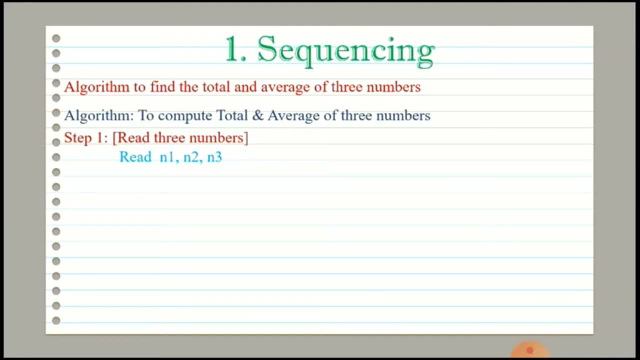 So after taking three inputs, we have to process that input. So in the step two we will calculate the total of three numbers and that result will be stored in total. So the statement will be read as n1 comma, n2 comma, n3 and the result will be stored. 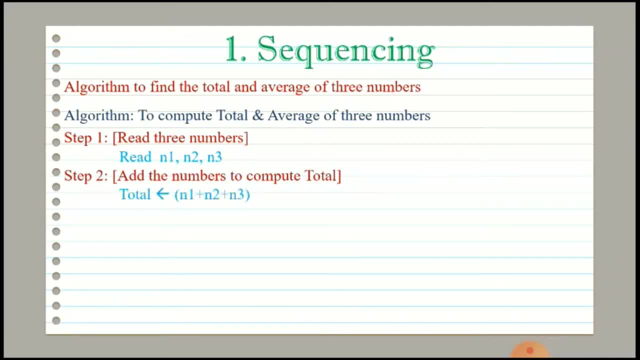 in total. So this is the result of the calculation and the result will be total equal to n1 plus n2 plus n3.. So after calculating total, now we can calculate average of that three numbers. So in step three we will take the total calculated in step two and divide that total by three. 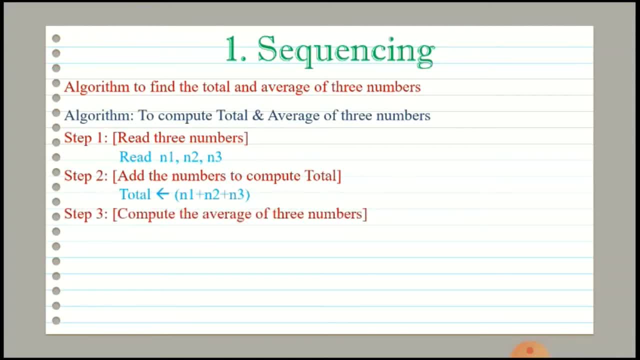 that you will get the average and save that result in the average. so the statement will be: average equal to total divided by 3. so after getting the total and average we have to print that result. so in step 4 we will print the total and average calculated in step 2 and step 3. so the 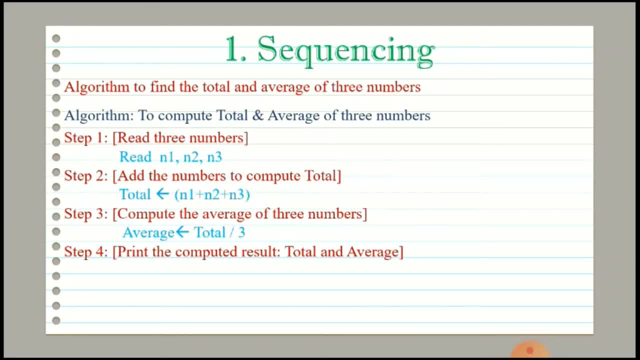 statement will be: write total comma average. the same statement. you can write it as print total comma average. so after taking input in first step and processing that input in second and third step and printing the result in fourth step, we have to stop the algorithm. so in fifth step, the statement. 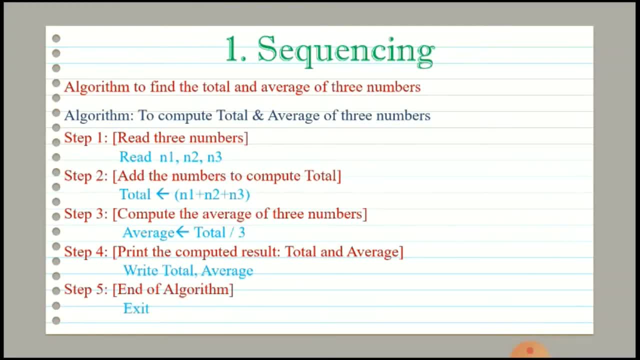 will be exit or you can write the statement stop. this will indicate that your algorithm is ended. so now we will take the values and, using algorithm, we will solve the given problem. suppose 22, 13 and 10 are the inputs. so this will be our first step. 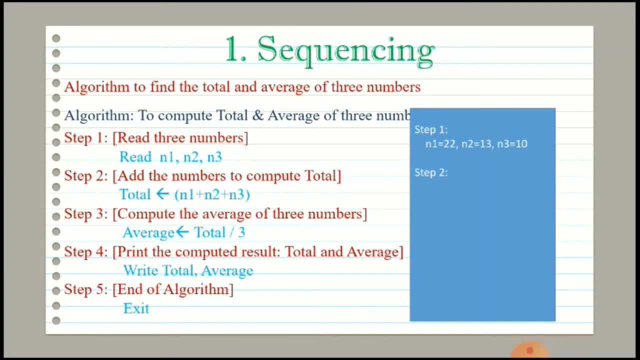 then in step 2 we will calculate the total by adding these three numbers and store that result in total. so the total is 45 and that will be stored in total. in third step we will calculate average. so divide total by three and save the result in average. so the average is 15 and that will be stored in average. 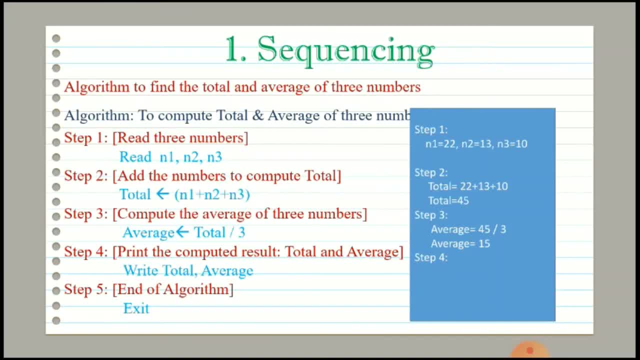 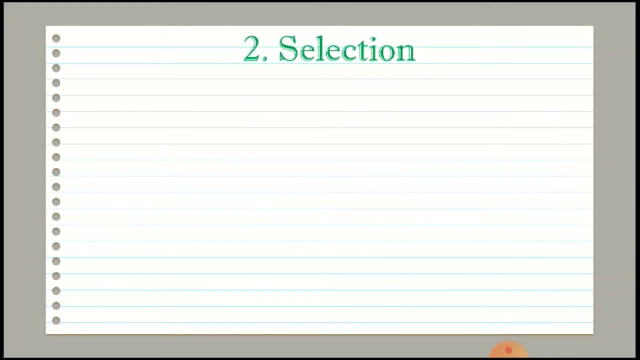 so after calculating total and average, in fourth step we will print the output. so print the output that is 45 and 15.. so after printing the output, in fifth step we will stop the algorithm by writing statement: stop or exit. so the second type is selection algorithm. selection algorithm defines conditional program. 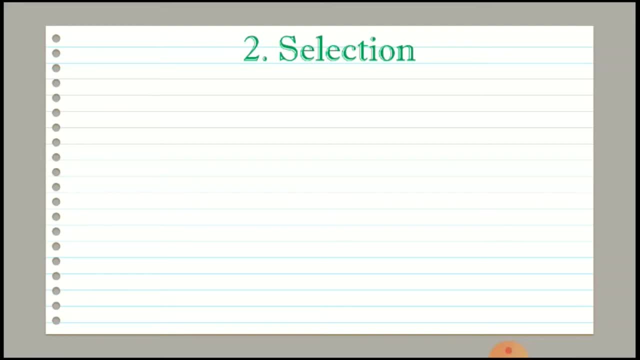 flow. the path of execution is selected depending upon whether a condition is true or false. so in selection algorithm the condition will be checked and depend on condition. if the condition is true, then the first statement will be executed and other statement will not execute, and if the condition is false, then second statement will be executed and first statement will not be. 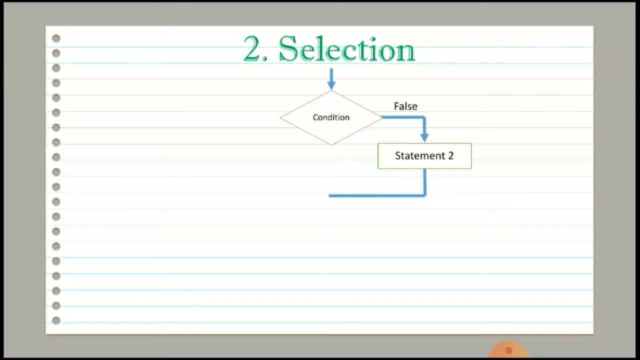 executed and first statement will not be executed. to understand easily we will see one example. the given problem is to find the largest number between two numbers. so here in here, if we write the new problem in the na provides the same cold condition, we will call it w so that as E is equal to 0, we have to change the format through. 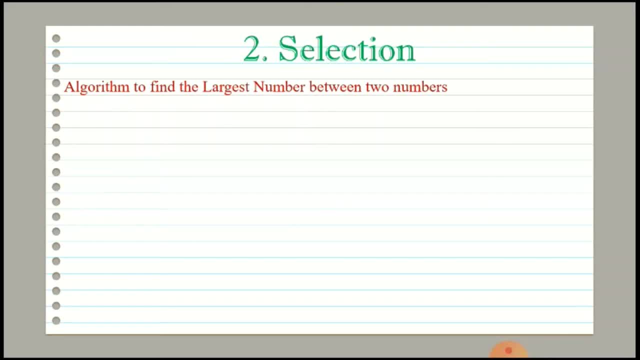 logical delet False. then to place n as v, we will. Here we have to find which number is largest between two given numbers. So here two numbers will be our input and checking the condition: which number is largest is the processing part, and displaying which number is largest is the output. 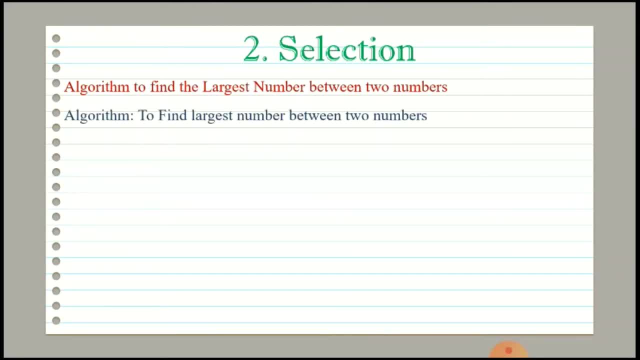 So the title of algorithm will be to find largest number between two numbers. Then in first step we have to read two numbers, So the statement will be Read. So in step two we have to check whether number is largest. Here we will compare two numbers. 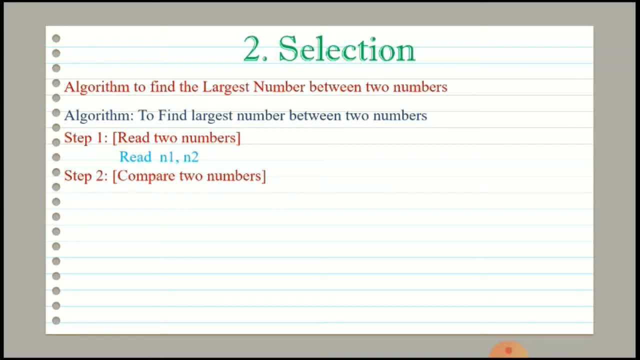 So if first number is largest, then second, then we have to save the value of first number in large, And if second number is largest, Then we have to save the value of second number in large. So in step two the first statement will be: if n1 is greater than n2.. 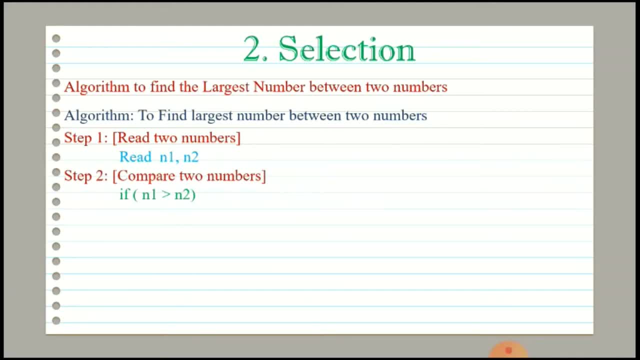 So here we are checking whether first number is larger than second number, And if this is true, Then we will save the value of n1.. In the Next step we have to find which number is largest between two numbers. So in step two we have to read two numbers. 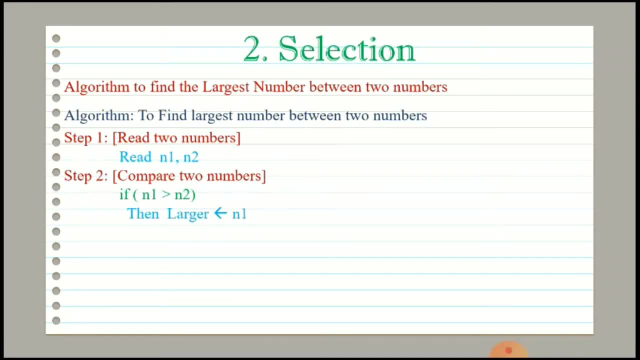 So here two numbers will be large, That is, large equal to n1. And suppose if n1 is not larger than n2. Then we will save the value of n2 in large And the statement will be else: large equal to n2.. 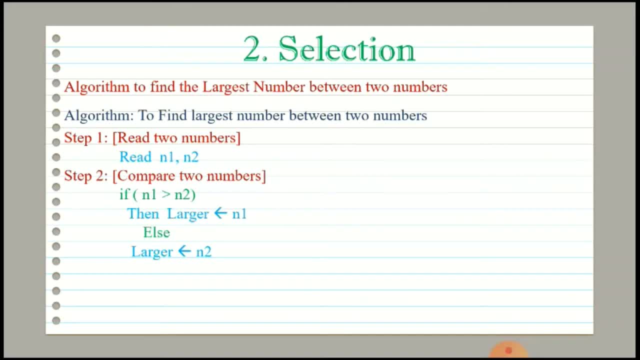 So if you see the statements written in step two, Depend on whether the condition is true or false, Only one statement will execute That is either large equal to n1 or large equal to n2.. So if condition that is n1 is greater than n2 is true, 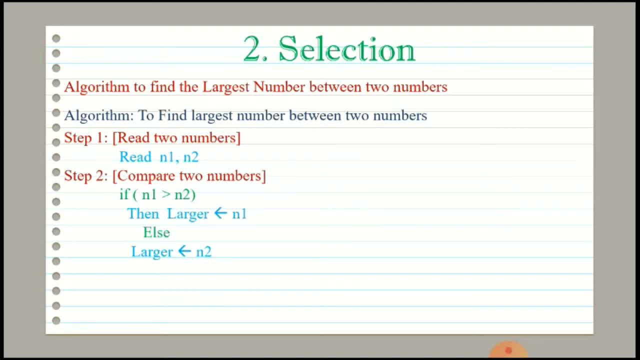 Then statement large equal to n1 will execute, And if condition that is n1 is greater than n2 is true, Then statement large equal to n1 will execute, And if condition that is n1 is greater than n2 is false, Then the statement large equal to n2 will execute. 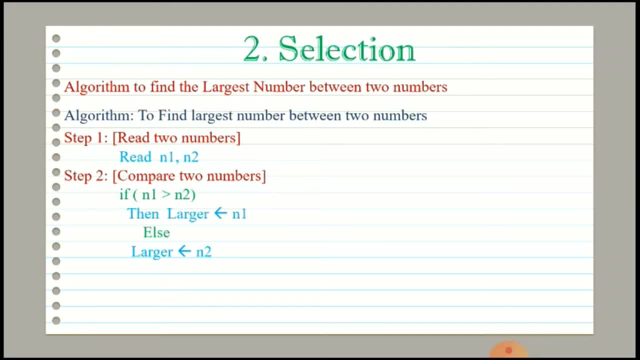 So after getting the result we have to print the result which is saved in large. So in step three we will print the result That is write large. So after reading the input in first step, we have checked which number is largest. in step two, 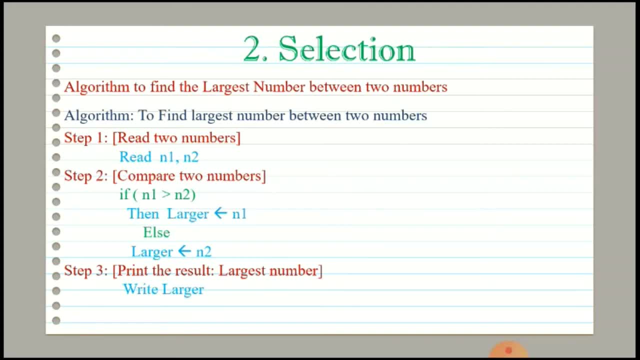 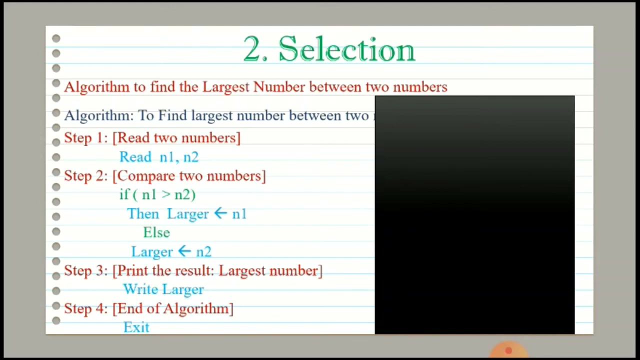 And in step three we have displayed the largest number. So in step four we have to stop the algorithm And the statement will be exit Now. Next, Now we will see the example by using the values and applying those values in algorithm. Suppose 20 and 30 are two numbers. 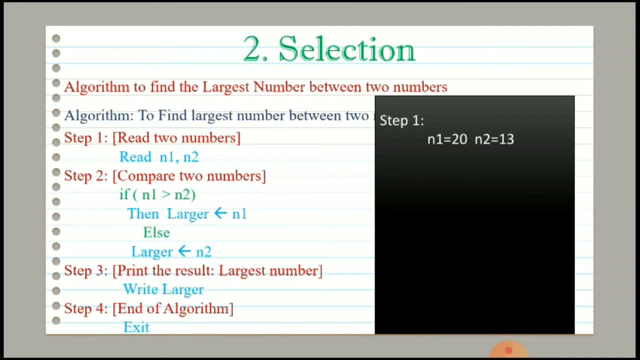 So this will be our first step. In step two we will compare these two numbers. So we will check whether n1 is greater than n2.. So we will check whether n1 is greater than n2.. So we will check whether n1 is greater than n2.. 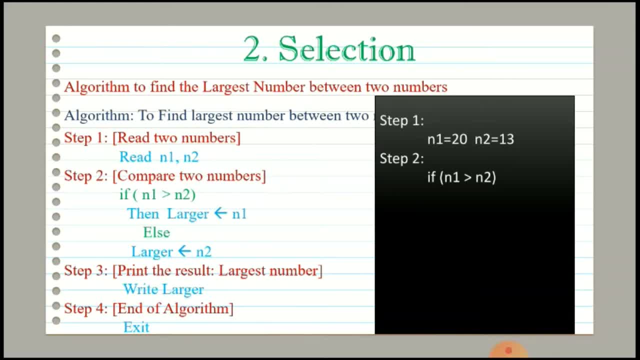 So in this case n1 is larger than n2, that is, 20 is greater than 13.. So we will save the 20 in larger. So we will see. So after getting the result in step three, we will print the result, that is 20.. 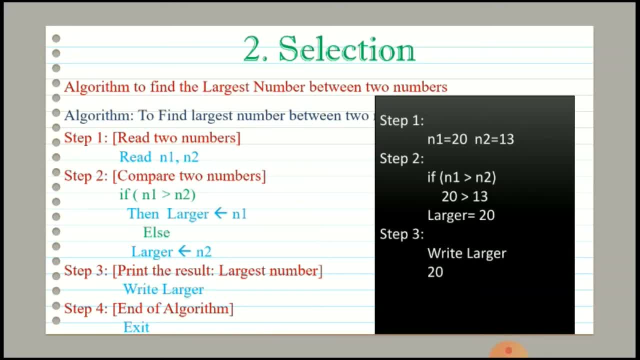 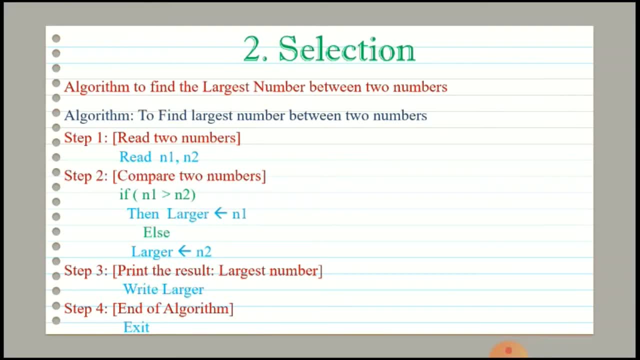 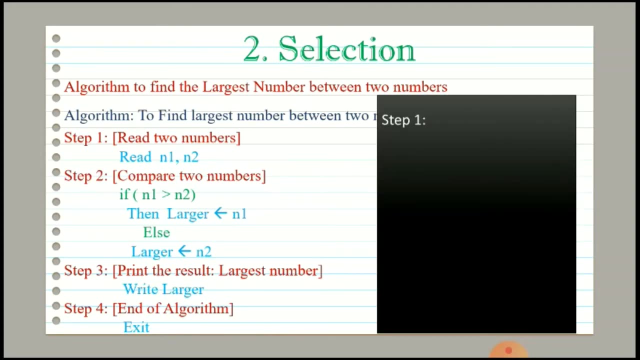 That is b 20.. step 4: we will stop the algorithm. we will see another example. suppose 15 and 27 are the two inputs. so this will be our first step. in step 2 we will compare these two numbers. so we will check whether n1 is greater than n2. so in this case n1 is. 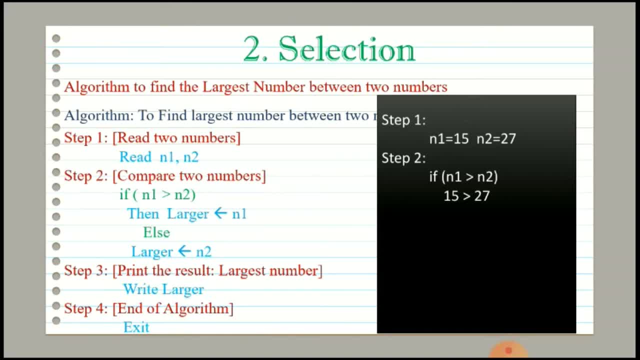 not larger than n2, that is, 15 is not larger than 27. so here we will save the value of n2 in large, that is, we will save the 27 in larger. so after getting the result in step 3, we will print the result. that is: 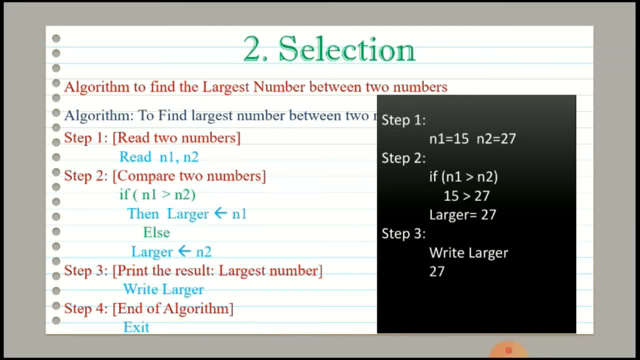 write larger and the value is 27. in step 4 we will stop the algorithm by writing exit. we will see one more example. suppose 25 and 25 are the two inputs. so this will be our first step. in step 2 we will compare these two. 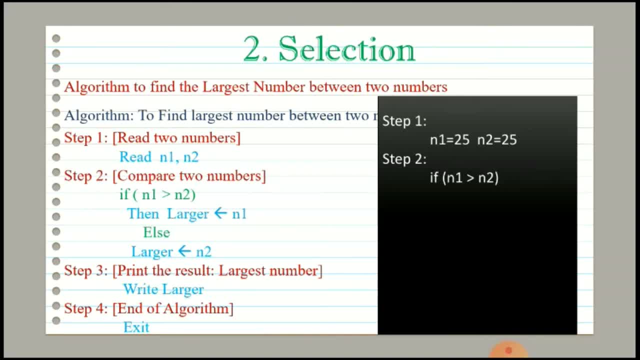 numbers. so we will check whether n1 is greater than n2. so in this case n1 is not larger than n2, that is, 25 is not larger than n2. that is, if 25 is not larger than n2, then n1 will be greater than n2. 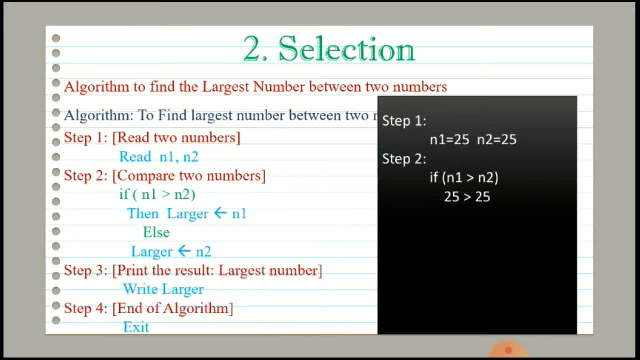 than 25. so here we will save the value of n2 in larger, that is, we will save 25 in larger. so after getting the result in step 3, we will print the result that is 25. in step 4 we will stop the algorithm. so if you see this example, both n1 and n2 are 25. 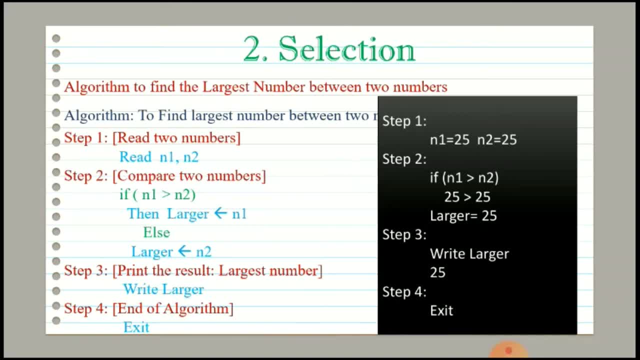 that means both the numbers are equal, but, as per our given problem, we are finding the largest value. so even both n1 and n2 are equal. so, if you see this example, both n1 and n2 are equal. so even both n1 and n2 are equal. so even both n1 and n2 are equal. so even both n1 and n2 are equal. 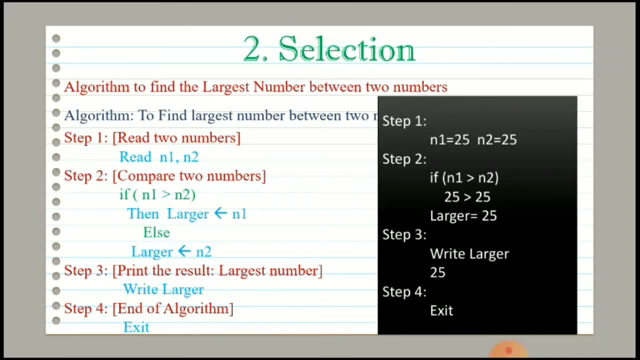 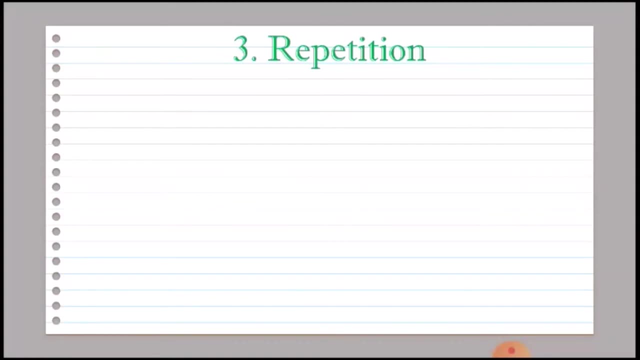 but the largest value is 25 itself. so the result is 25 repetitive. in repetitive algorithm, repetitive execution of statements takes place as long as condition is true. the moment when the loop condition becomes false, the loop or repetition will be stopped. so in repetition algorithm the condition will be checked and depend on. 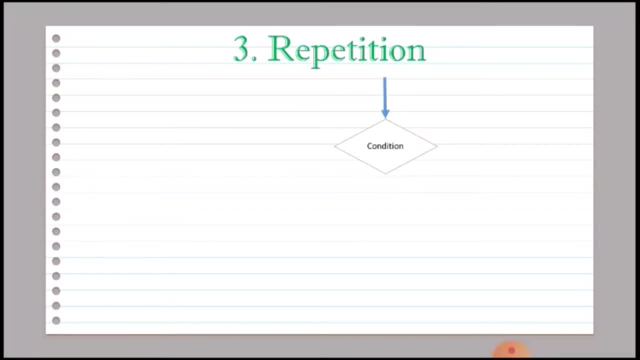 condition. if the condition is true, then the statement will be executed and this statement will be executed continuously till the condition is true. the moment when the condition becomes false, it will stop executing those statements and it will move to the next step. to understand repetitive algorithm easily, we will see one example. the given problem is to calculate. 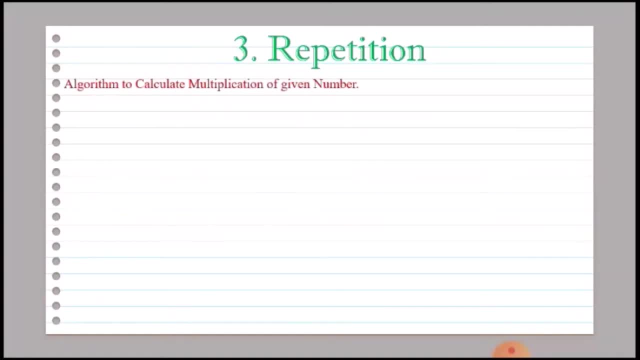 the multiplication table of given number. so here we have to find the multiplication table of a given number. so here a number whose multiplication table you want will be our input, and calculating the multiplication table of a given number is the processing part, and displaying the multiplication table is the output. 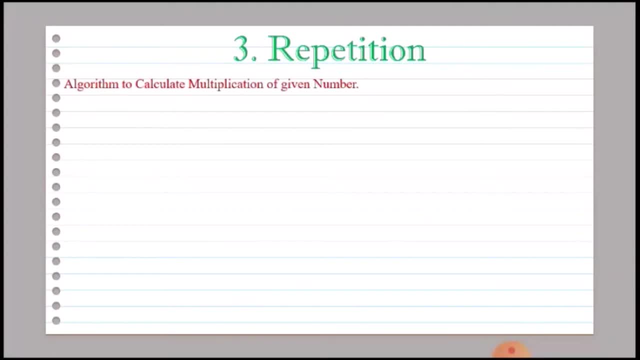 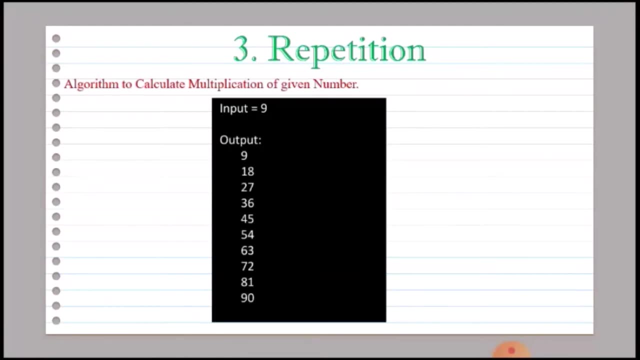 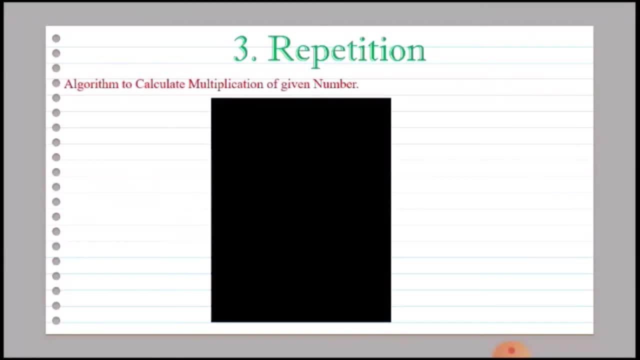 multiplication 10 times. so suppose you are finding the multiplication table of 9, then the first output is 9, that is 9 into 1. the second output is 18, that is 9 into 2. the third output will be 27, that is 9 into 3. the fourth output is 36, that is 9 into 4. the fifth output will be 45, that is 9 into 5. 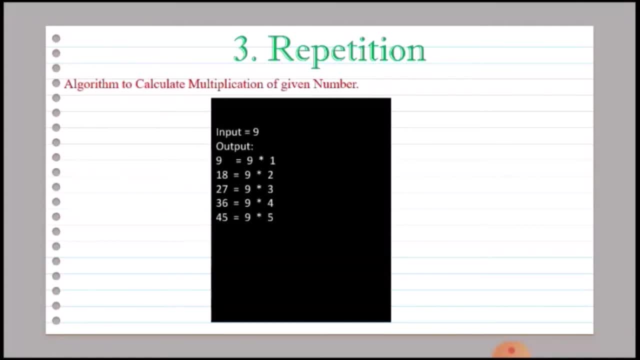 the sixth output will be 54, that is 9 into 6. the seventh output will be 63, that is 9 into 7. the 8th output will be 72, that is 9 into 8. the 9th output will be 81, that is 9 into 9, and the 10th output will be: 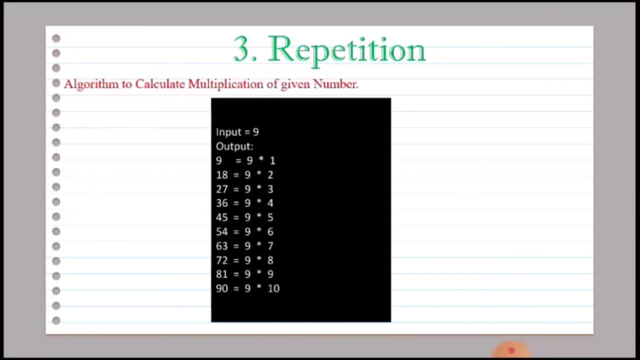 90, that is 9 into 10. so if you see the output, you have to repeat the same multiplication 10 times by using 9 and other value by increasing that value by one. so first we will multiply 9 by 1, then 9 by 2, and then years 9 times 3, and so on. 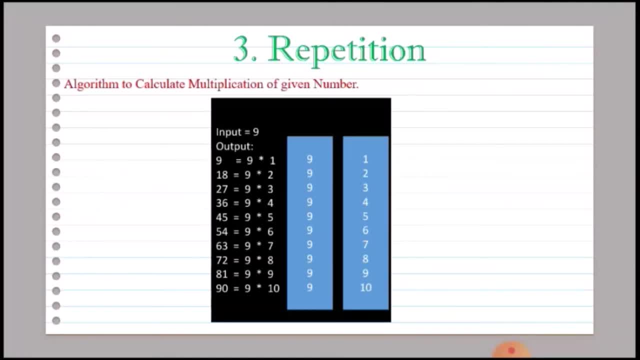 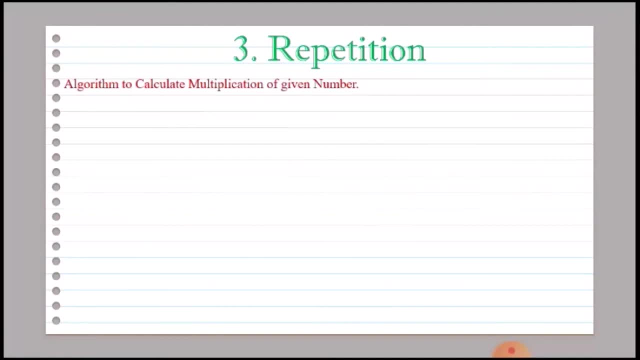 in the term to the last multiplication, that is 9 times 10. So the title of algorithm will be to calculate the multiplication table of a given number. So in first step we will initialize the count by 1.. That is, count equal to 1.. 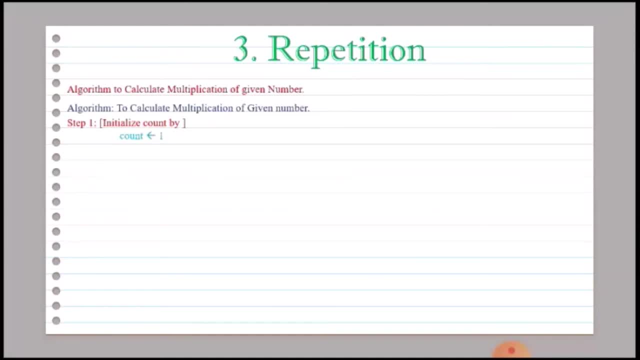 This count is used to multiply the given number and after multiplying we will increase the value of count by 1 to perform next multiplication, and so on. So basically, We will increase the value of count by 1, 10 times to get the required output. 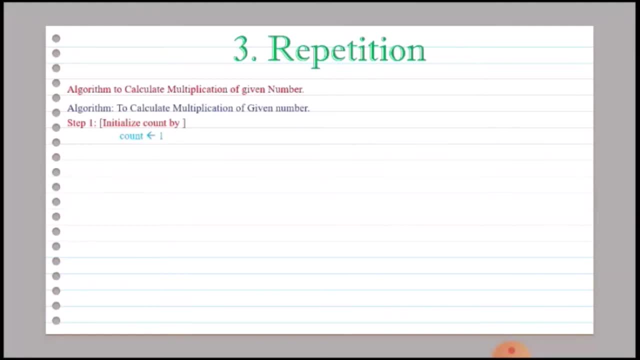 Then in second step we have to read a number, So the statement will be read n. So in step 3 we have to calculate multiplication. So we will multiply n by count And we will store the result in multiplication. So the statement will be: multiplication equal to n into count. 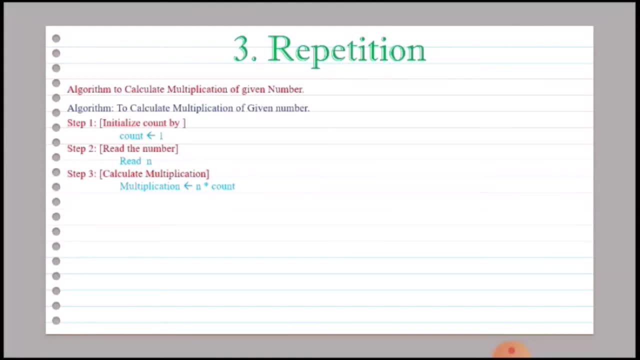 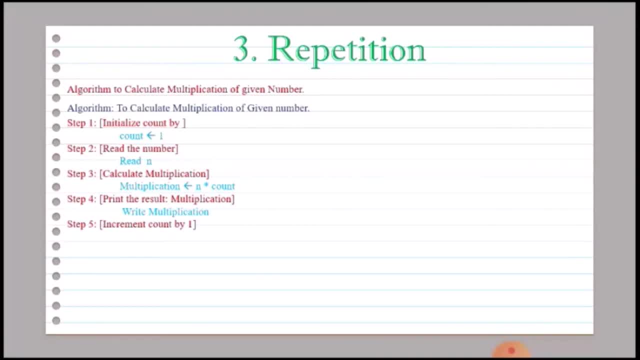 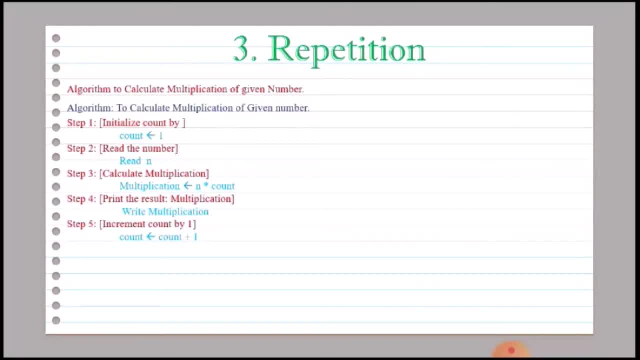 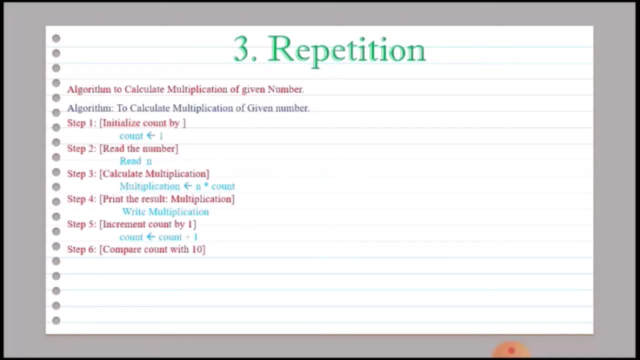 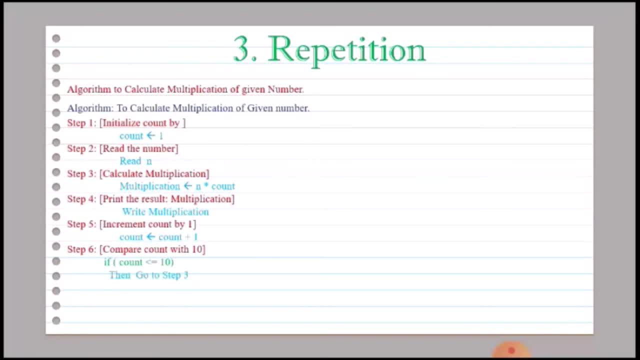 Write n, Write n. So the statement will be go to step 3.. If you see this statement, if the condition is true, then we are going again back to the third step. So basically, we are repeating the previous steps again which we have already executed. 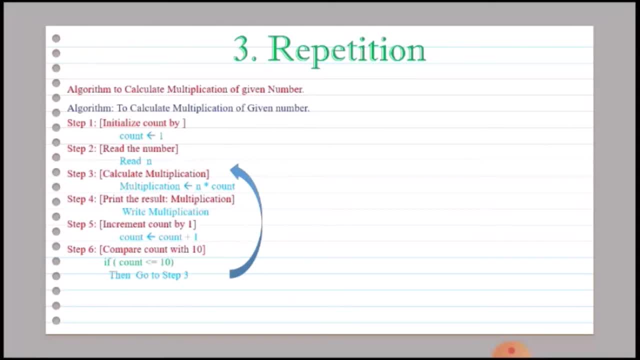 So in this case, if condition is true, then we will go back to the step 3 and we will start from step 3 again. So in step 3, the statement is multiplication equal to n into count. So now we will multiply n by count and the value of count is 2.. 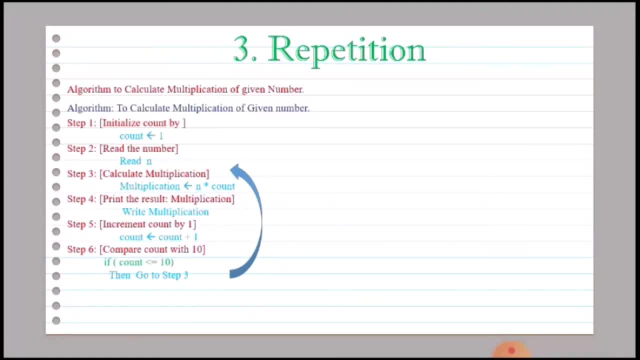 So the result will be saved in multiplication and next we will move to the Step 4.. So in step 4 we will print the value of multiplication. So after printing we will go to the step 5.. So in step 5 we will increment the value of count by 1.. 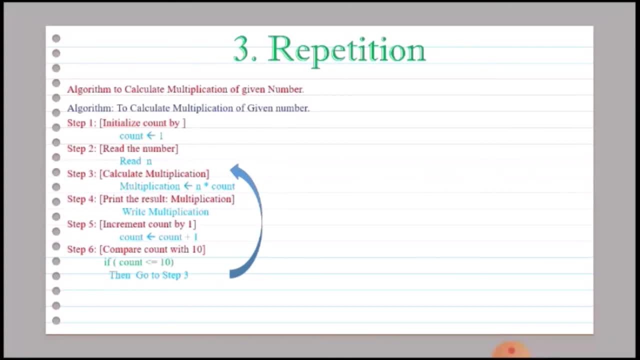 Now the value of count becomes 3.. After incrementing The Houma m, A value of count, we will go to the step 6. so in step 6 we will compare count with 10. so if this condition is true, then we will again go back to the step 3. so this: 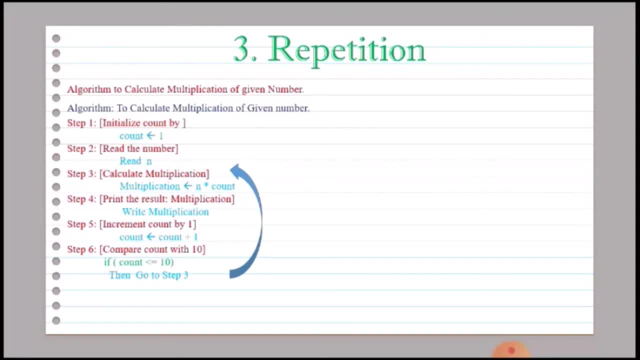 same process will be repeated 10 times. after 10 times repetitions condition becomes false, so the statement will be: else: go to the step 7. so now we have got the output and also printed that output. so in step 7 we have to stop the algorithm. 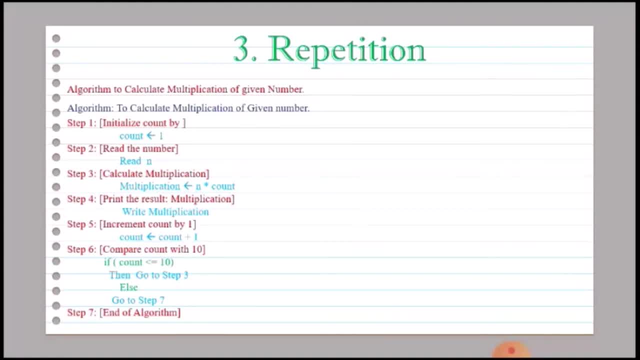 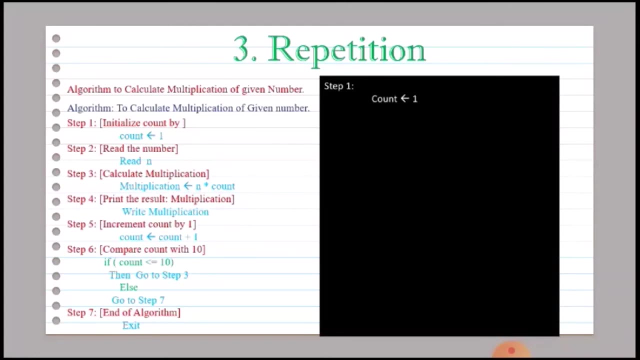 so the statement will be exit. now we will take the values and see how the algorithm works. so in step 1 we are assigning the value 1 to the count. in step 2 we will read the value of n. suppose the value of n is 12. so in step 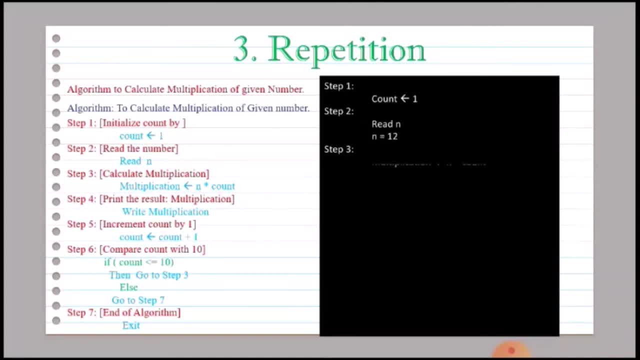 Step 3 we will multiply n by count. So the value of n is 12 and the value of count is 1.. So 12 into 1 is 12 and that result will be saved in multiplication. In step 4 we will print the result saved in multiplication. 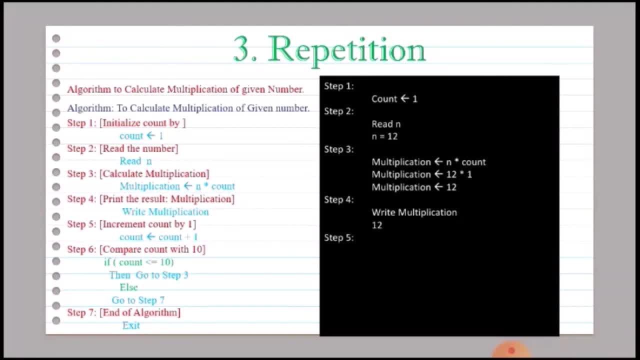 So we will print 12.. In step 5 we will increment count by 1. So now count will become 2.. In step 6 we will check whether count is less than or equal to 10. So in this case count is 2.. 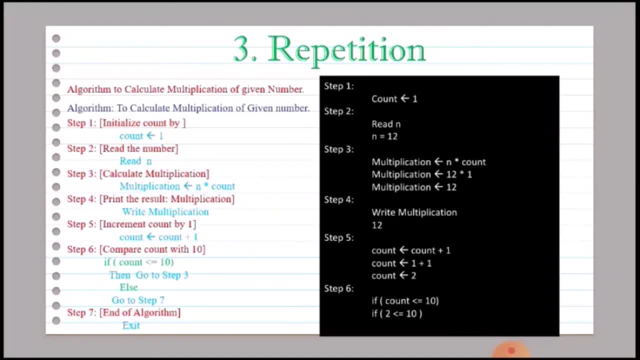 And 2 is less than or equal to 10, which is true. So if the condition is true, then we will go back to the step 3.. So in step 3 we will multiply n by count. n is 12 and count is 2.. 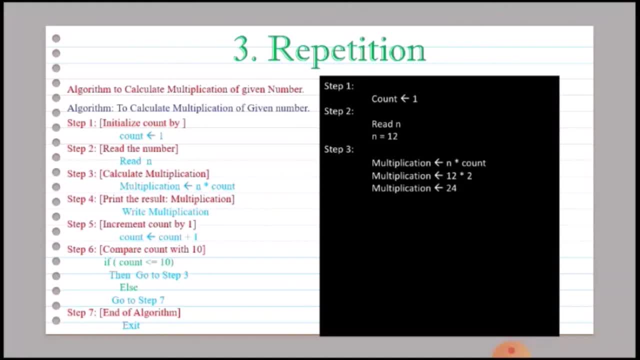 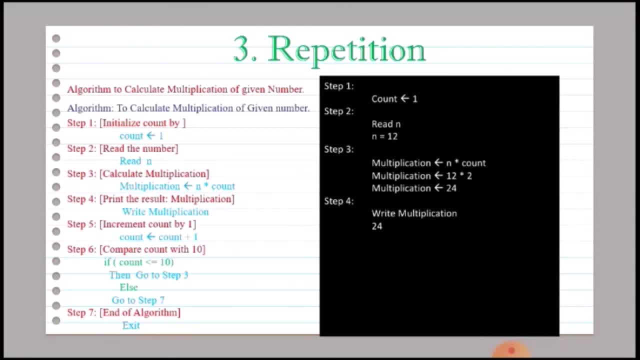 So in step 4 we will print the 24. In step 5 we will increment count by 1. So now count will be 3.. So now count will be 3.. In step 6 we will check whether count is less than or equal to 10.. 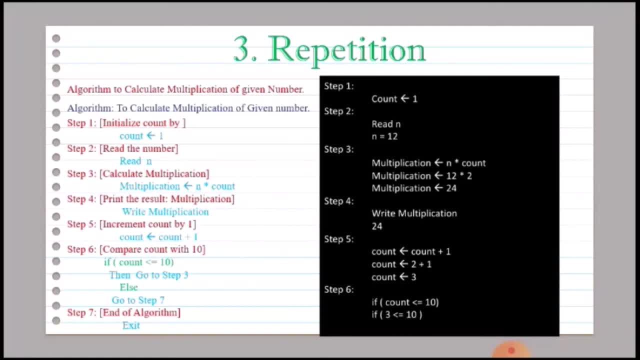 So in this case count is 1.. count is 3 and 3 is less than or equal to 10, which is true. So if the condition is true, then we will go back to the step 3 again. So in step 3 we will multiply n by count. 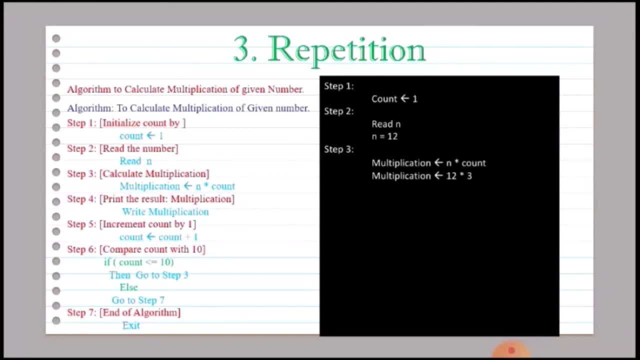 So n is 12 and count is 3. So the answer is 36. So in step 4 we will print the 36. In step 5 we will increment count by 1. So now count will become 4.. Step 6: we will check whether count is less than or equal to 10.. 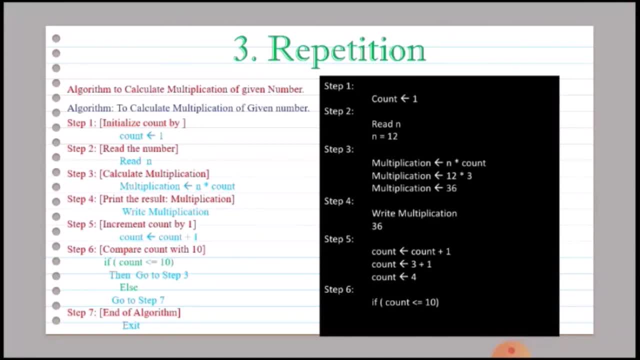 So if 4 is less than or equal to 10, which is true. So if the condition is true, then we will go back again to the step 3.. So in step 3 we will multiply n into count. So 12 into 4 is 48.. 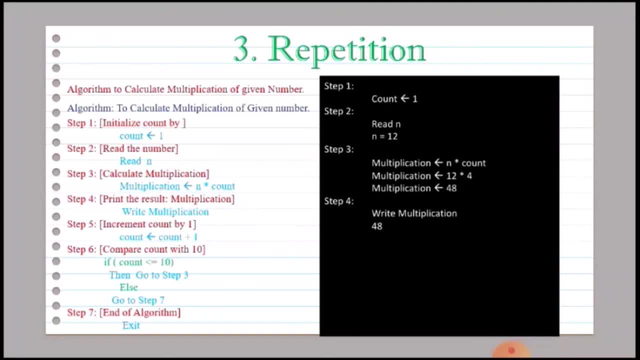 So in 4th step we will print 48.. So in step 5 we will increment count by 1. So now count will become 5. So in step 6 we will print 48.. So in step 5 we will print 48.. 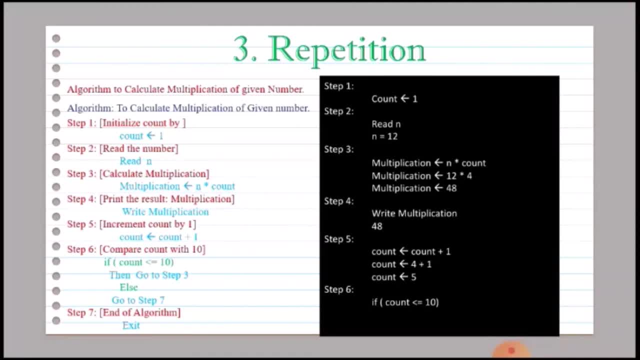 So in step 6, we will increment count by 1.. So in step 6, we will check whether count is less than or equal to 10.. So we will check whether 5 is less than or equal to 10, which is true. 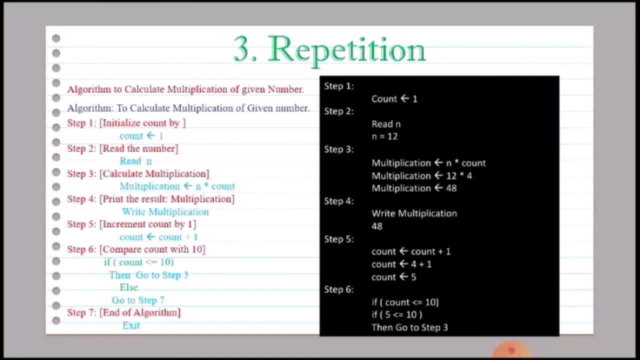 So if the condition is true, then we will go back to the third step again. So in step 3 we will multiply n by count. So in 2nd step we will print 48. So n is reduced by 4. So n is 12 and count is 5.. 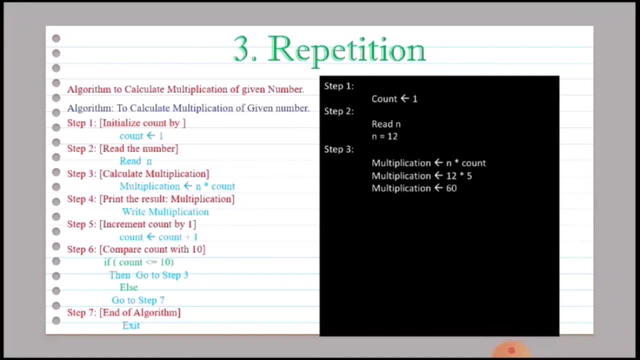 So the answer is 60.. So in step 4 we will print the 60. Step 5, we will increment count by 1.. So in step 5 we will increment count by 1. So now count will become 6.. 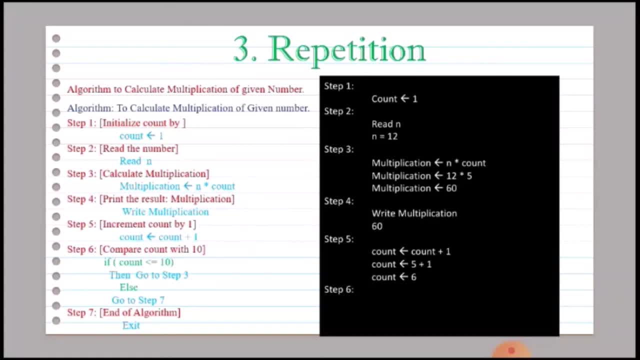 In step 6 we will check whether count is less than or equal to 10. So in step 8 we will print the 90. So in step 8 we will print the 90. So in step 9 we will show that count by 1.. 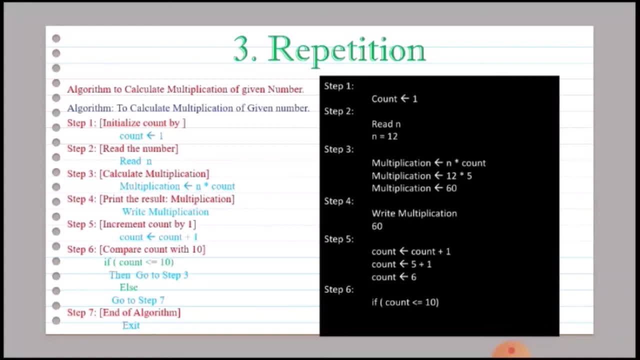 check whether count is less than or equal to 10. so in this case count is 6 and 6 is less than or equal to 10, which is true. so if the condition is true, then we will go back to the step 3. so in step 3 we will multiply n by count. n is 12. 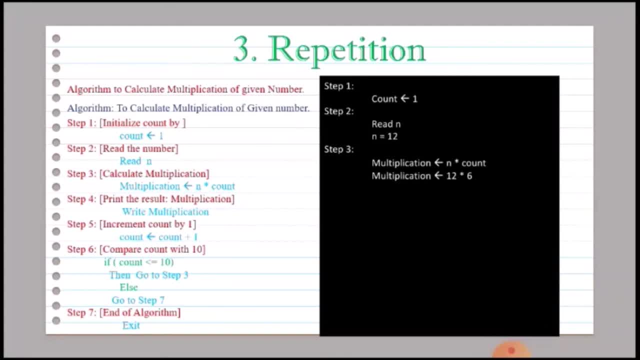 and count is 6, so the answer is 72. so in step 4 we will print the answer, that is 72. in step 5 we will increment count by 1, so now count will become 7. in step 6 we will check whether count is less than. 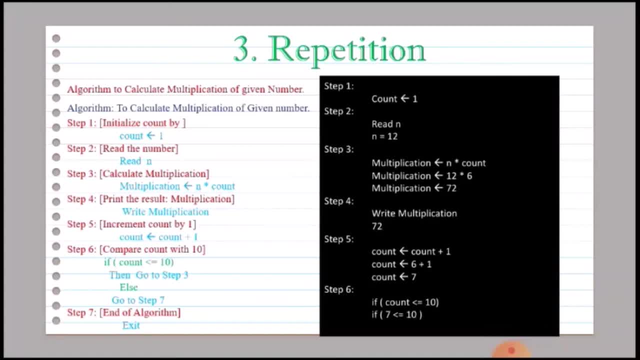 7. in step 6 we will check whether count is less than or equal to 10. so in this, In simple metaphor, you are able to compute the policy in equations or observations. or equal to 10. so in this case count is 7 and 7 is less than or equal to 10, which is true. so if 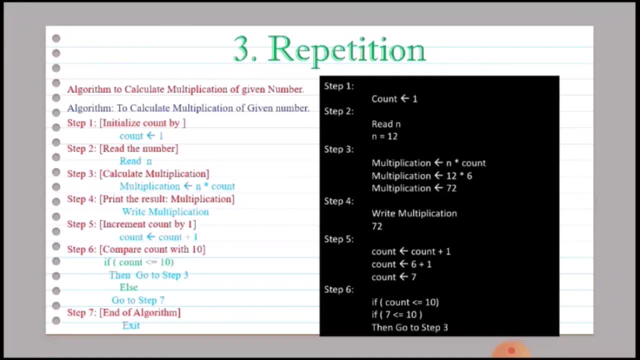 the condition is true, then we will go back to the step 3 again. so in step 3 we will multiply n by count. so n is 12 and count is 7, so the answer is 84. so in step 4 we will print 84. 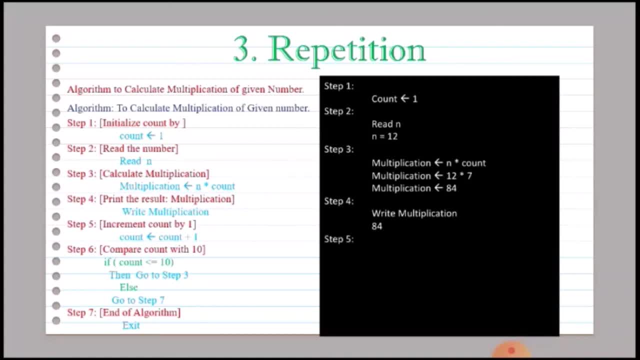 84. so in step 5 we will increment count by 1, so now count will become 8. in step 6- 8- we will check whether count is less than or equal to 10. so in this case count is 8 and 8 is less than or equal to 10, which is true. so if the condition is true, 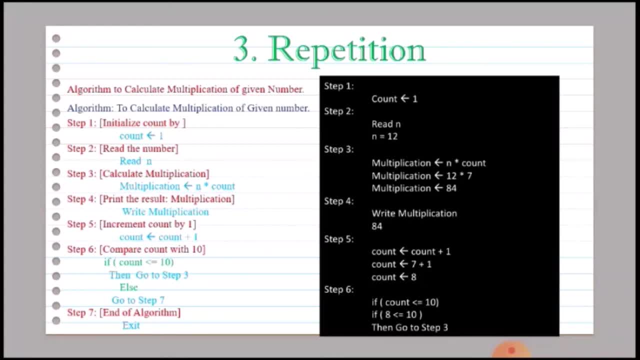 then we will go back to the step 3 again. so in step 3 we will multiply n by count. so n is 12 and count is 8, so the answer is 8. we will go back to the step 3 again. so n is 12 and count is 8, so the answer is beans. 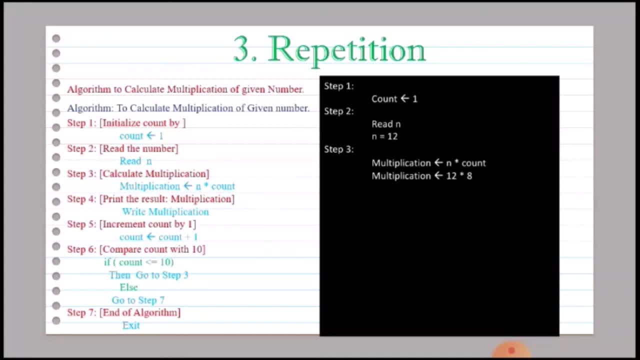 9 count. so n is 12 and count is 8. so the answer is Mahland: 4, 4. so n is 12 and count is 8. so the answer is cancer: 9, 5, 5, 4, 3, 3, 2. 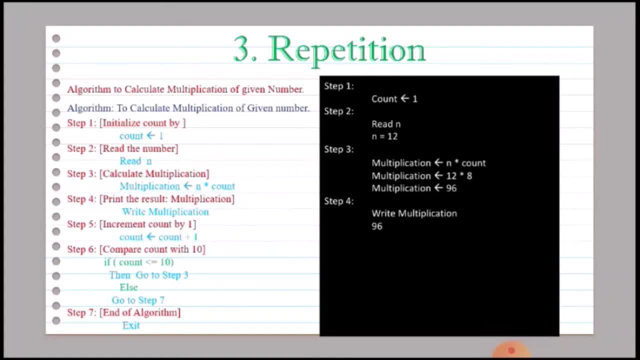 3, 3, 4, 3, 3, 3, 4, 4, 5, 5, 6, 6, 7, 3, 8, 6, 7. In step 6, we will check whether count is less than or equal to 10.. 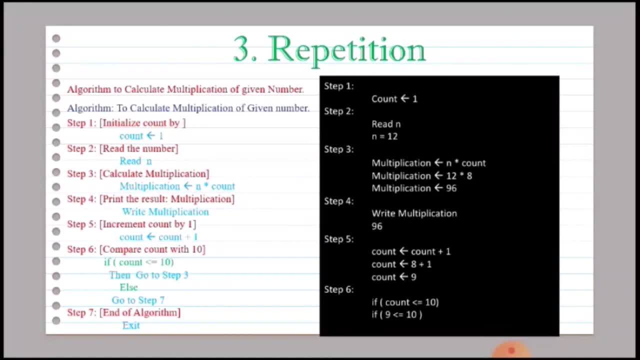 So in this case, count is 9 and 9 is less than or equal to 10, which is true. So if the condition is true, then we will go back to the step 3.. So in step 3, we will multiply count by n, and n is 12 and count is 9.. 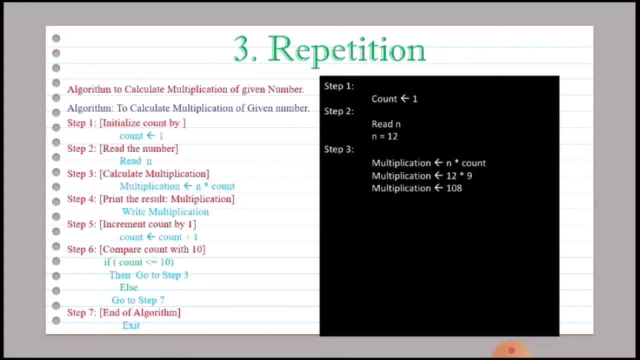 So the new answer of multiplication is 108.. So in step 4, we will print the answer that is 108.. In step 5, we will print the answer that is 108.. In step 6, we will increment count by 1.. 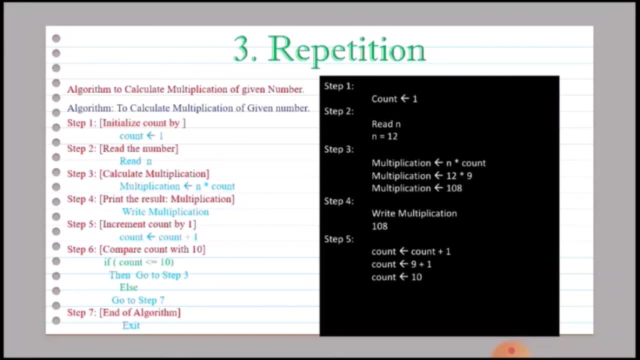 So now count will become 10.. In step 6, we will check whether count is less than or equal to 10.. So in this case, count is 10 and 10 is less than or equal to 10, which is true. 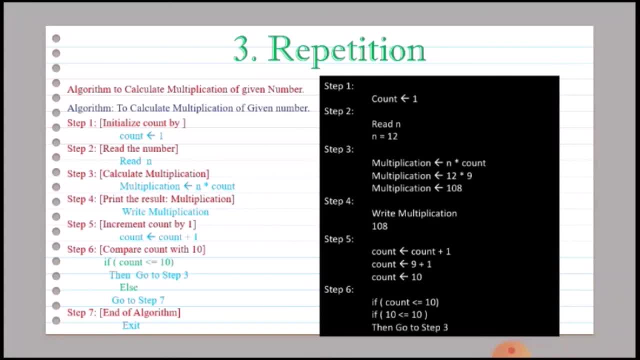 So if the condition is true, then we will increment count by 1.. So if the condition is true, then we will go back to the step 3 again. So in step 3, we will multiply n by count. n is 12 and count is 10..